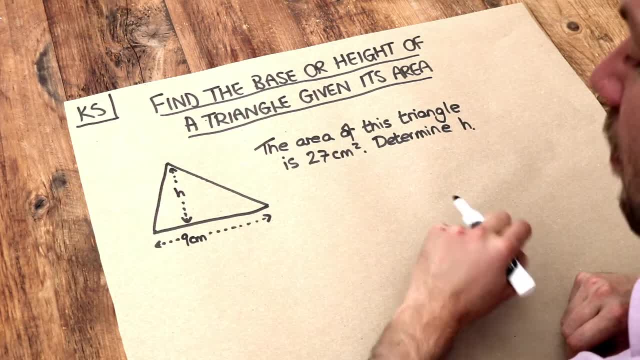 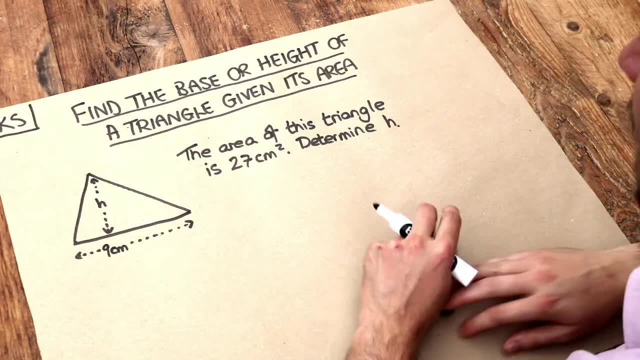 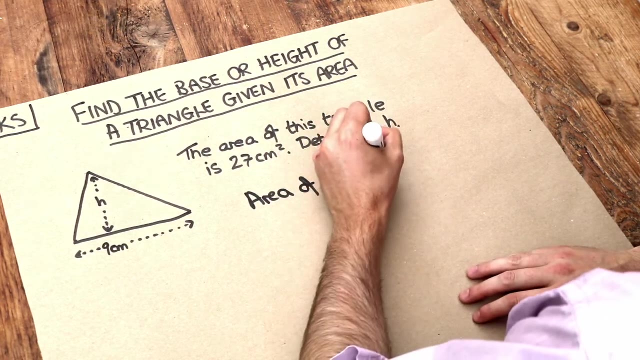 But now we're working backwards. We've got the area of the triangle and we've got either the base or the height, and we want to find either the height or the base, depending on which one we have. So let's remind ourselves of the area of a triangle formula: The area of a triangle is equal to the base. 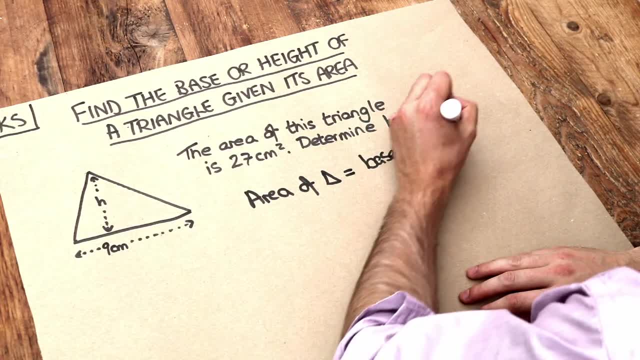 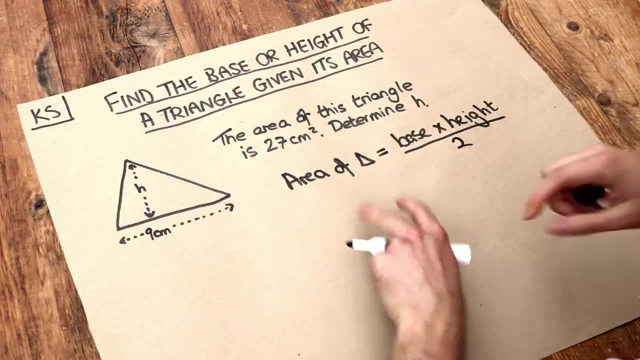 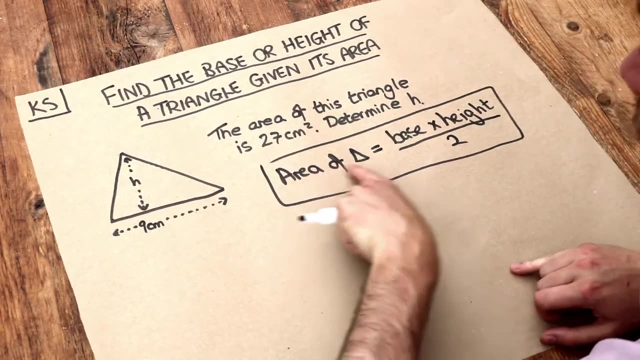 times the perpendicular height. So the height has to be at right angles to the base and we divide it by two. Now let's use this formula to plug in, to substitute what information we have in the question. We've got the area of the triangle, that's 27,. 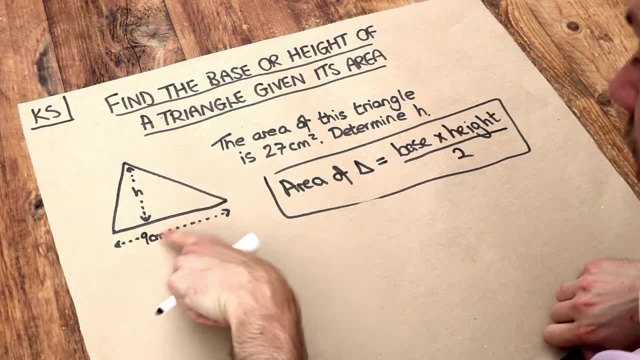 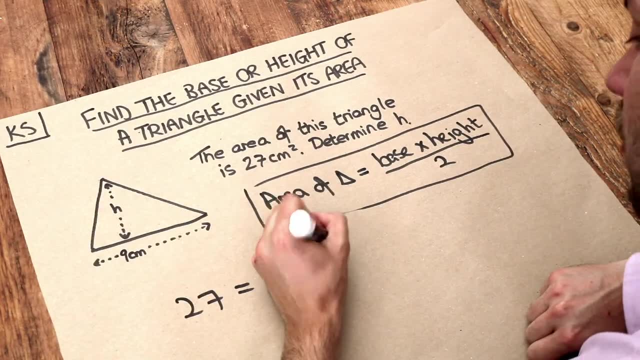 and that is equal to the area of the triangle. So that's equal to the base of the triangle, which we know is 9, multiplied by the height of the triangle, which is h, And remember that height has to be at right angles to the base. 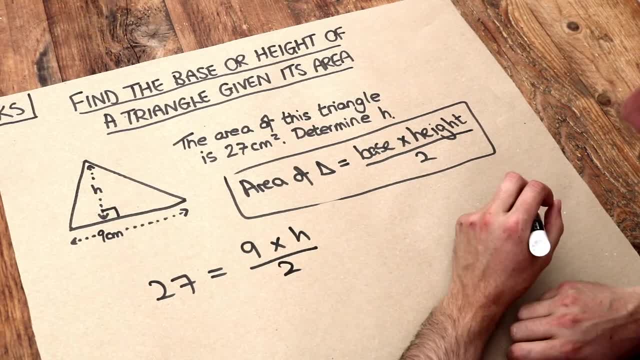 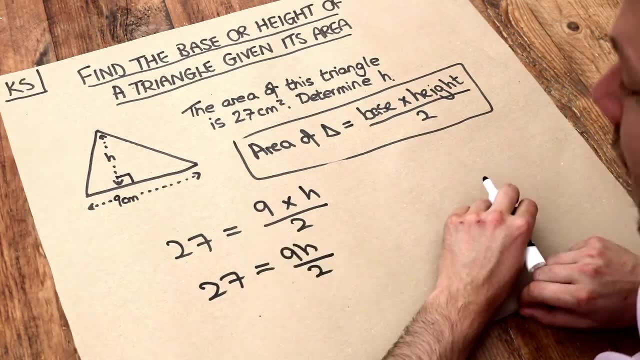 And then we can see there's a divide by two. So we just need to solve this equation. Now, if I just simplify this: 9 times h is just 9h. Now how would we solve an equation like this? We want to try and get h on its own. 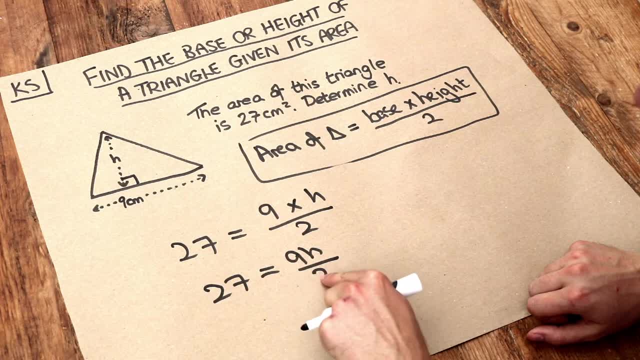 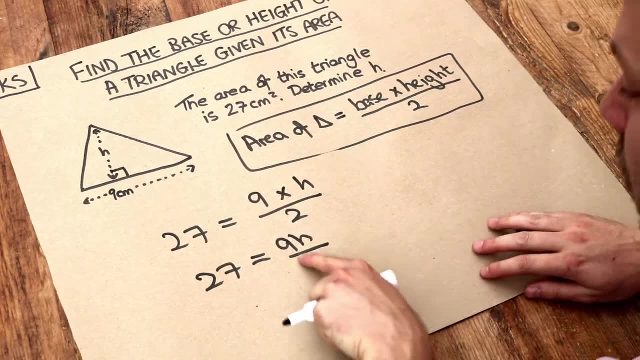 And we can see that h has been multiplied by 9, and divided by 2.. Now remember we want to undo the last thing that happened to the variable vh first, So we want to undo get rid of that over 2.. What's the opposite of dividing by 2?? 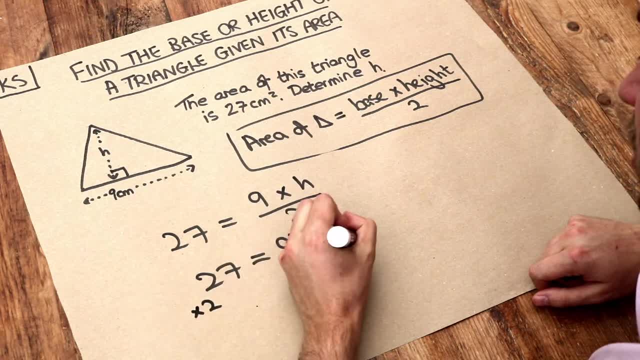 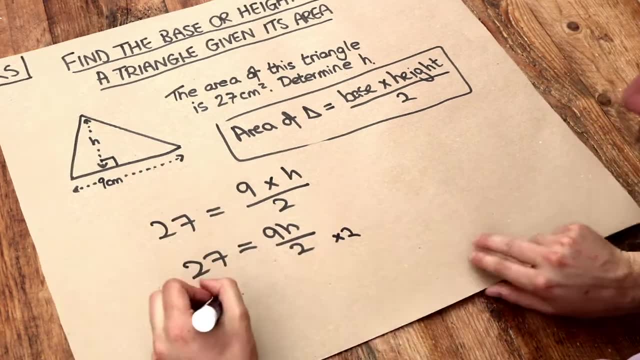 Well, it's timesing by 2.. So if we multiply both sides by 2, that's the opposite of dividing by 2, so it will get rid of that over 2.. So 27 times 2 is 54, and we're doing the same thing to the right-hand side. 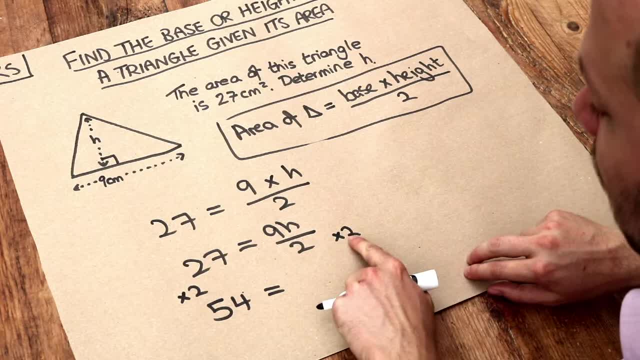 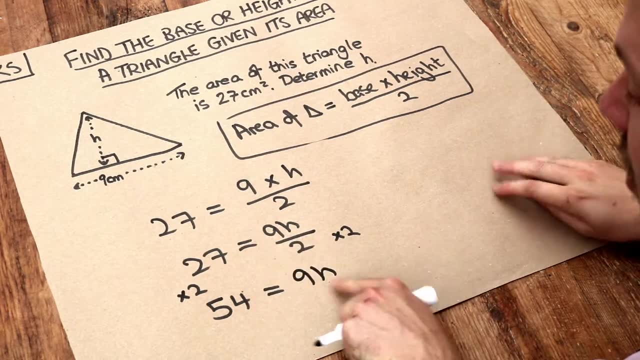 Whatever we do to the left-hand side, we have to do the same to the right-hand side. If we times by 2, that gets rid of it, cancels out that over 2, just leaving the 9h. Now the h is being multiplied by 9.. We want to get rid of that multiplied by 9.. 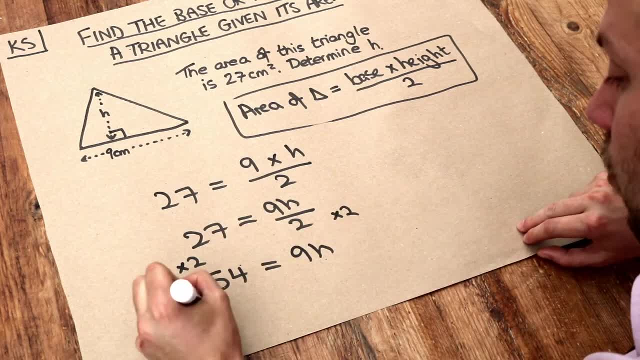 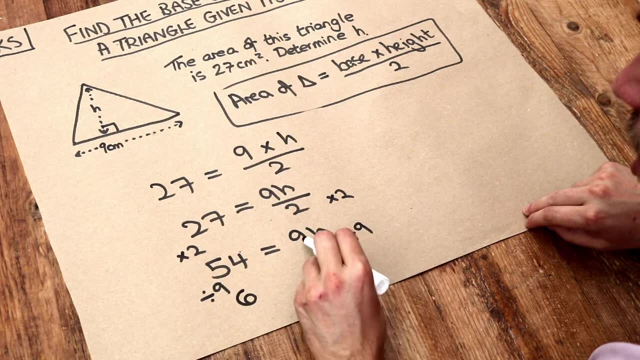 What's the opposite of multiplying by 9? Dividing by 9.. So, therefore, we divide both sides of the equation by 9.. 54 divided by 9 is 6. And 9h divided by 9,. well, the divide by 9 cancels out the times by 9, we just get h.